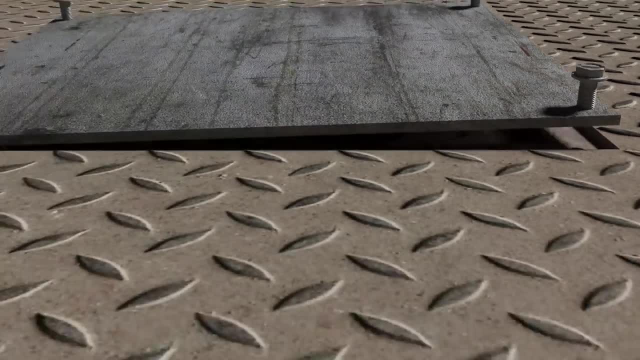 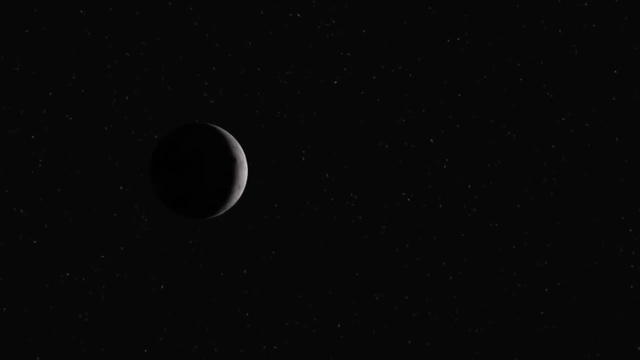 Each time you look at the moon, it's going to look a little different. Sometimes you'll see the entire moon, other times you'll see just a portion of it. In this video, I'd like to go over why the moon looks the way it does and a few other things about the moon's orbit. 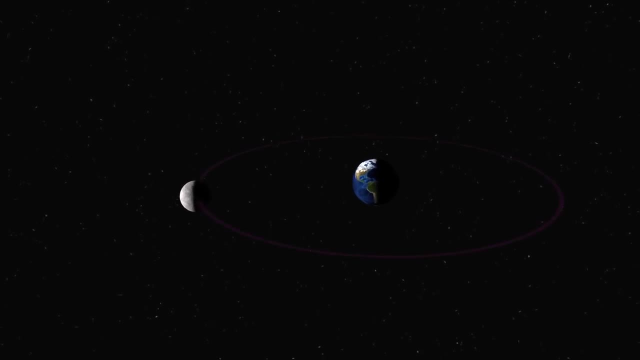 The moon takes about a month to orbit the earth. The sun can only shine on half the moon at any given time. Since the moon orbits at exactly the same rate as it spins, we only see one side of the moon from the earth. The side we don't see is usually called the far side of the moon. 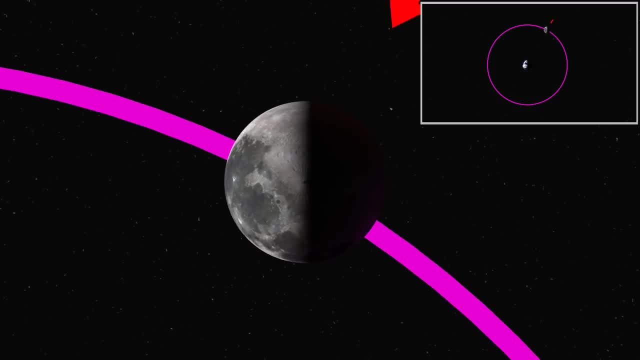 You can also call it the dark side of the moon, but it's not always dark, so this name can be a bit confusing. I'm going to show a split screen here to show you how it looks. I'll show things from two different views. 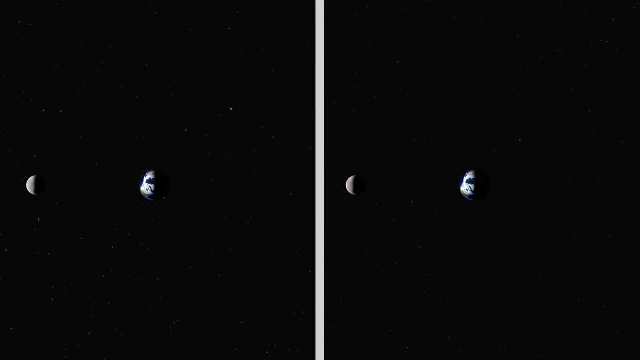 On the left-hand side of the screen, I'll show a top-down view. On the right-hand side of the screen, I'll show what it looks like from earth When the moon is closest to the sun. the side of the moon facing the earth is dark. 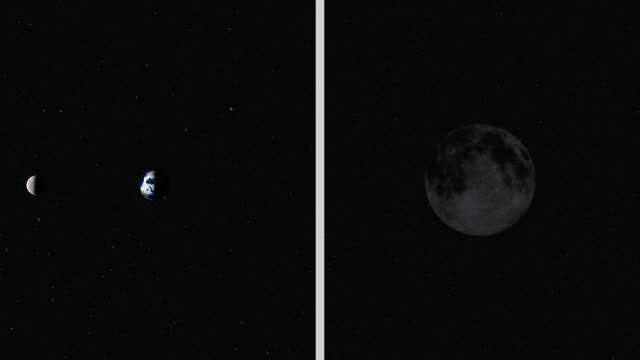 The sunlight reflects off the earth, so we can still see the moon if we look closely. We refer to this as a new moon. As the moon comes around, we start to see a tiny sliver of the moon. This is called the waxing crescent. 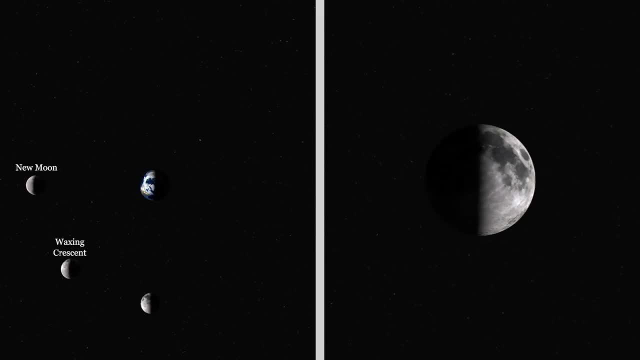 A few more days pass by and now we can see half the moon. We can call this a half moon, but more specifically it's called a first quarter, because we are a quarter of the way through the phases. A few more days and only a small portion of the moon is not lit up. 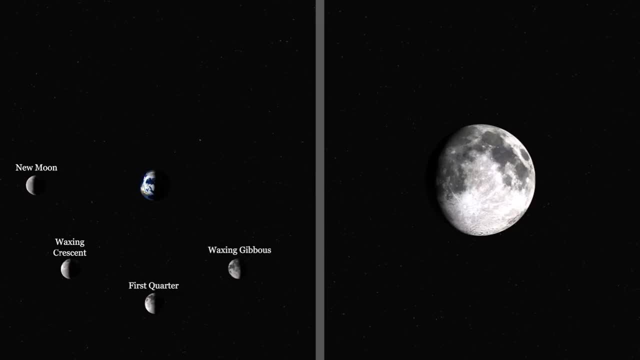 This is called the waxing gibbous. When the moon is on the other side of the earth, it is completely lit. This is called a full moon, and it's probably the phase that you're most familiar with. Now the light begins to fade.